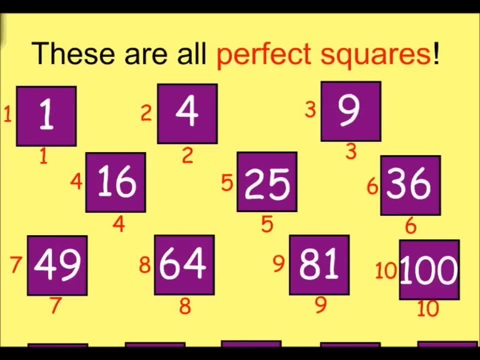 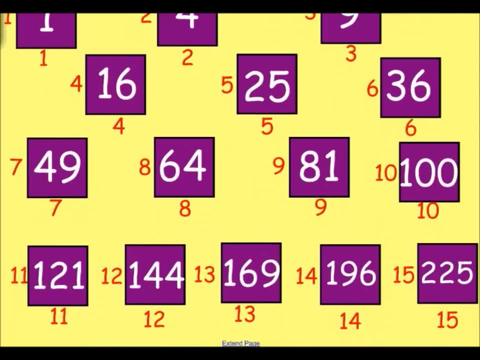 They all make squares. Here's just a few. Here's just a few more perfect squares. We've already done the ones to 100.. 11 times 11 is 121.. 121 is a perfect square: 12 times 12,, 13 times 13,, 169,, 196.. 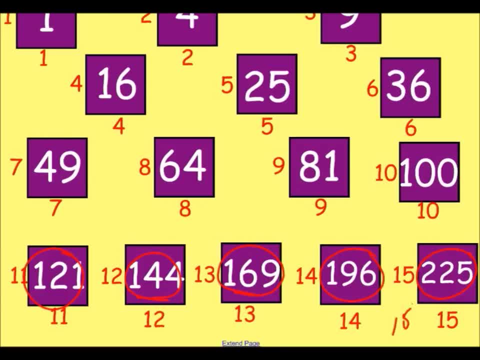 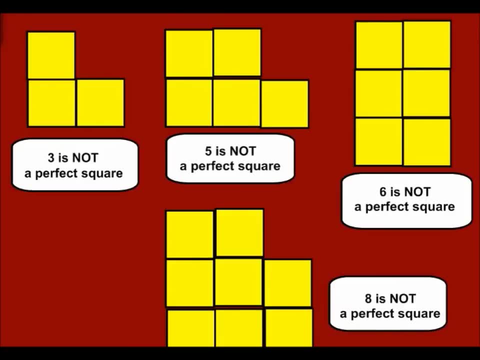 225 is a perfect square. 15 squared is 225.. 225 is a perfect square. Well, let's talk about what aren't perfect squares: 3.. 5 is not a perfect square. It doesn't make a square. 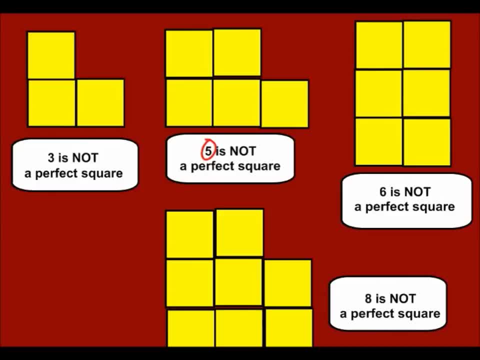 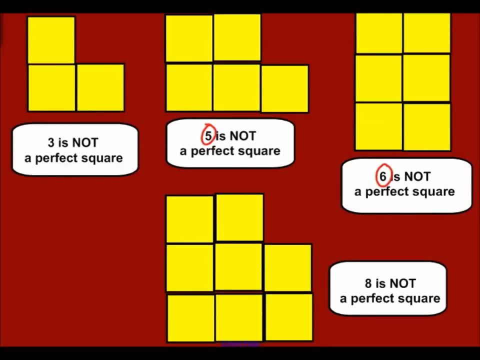 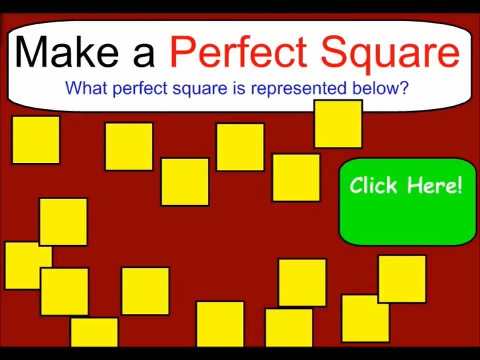 5 is also The number 5 is not a perfect square. It doesn't make a square. 6 is also not a perfect square And the number 8 is not a perfect square. Let's make a perfect square right here. 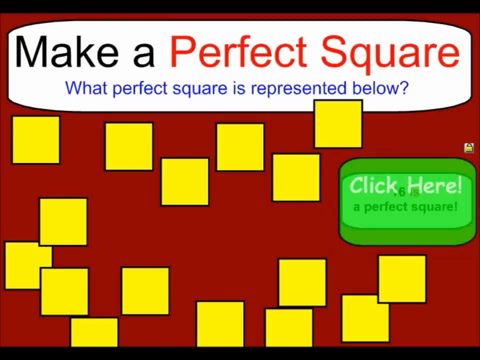 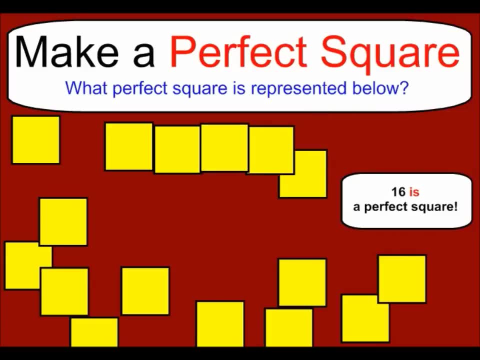 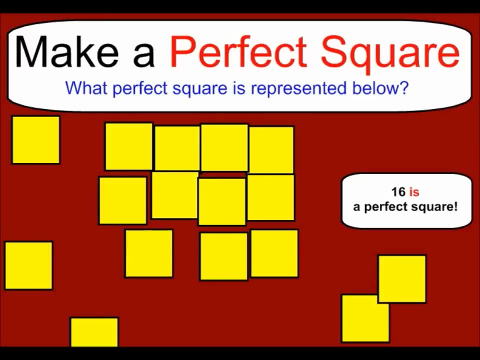 So what perfect square is represented below? Let's click here and find out 16.. It's a perfect square Because if we put these all together, the number 16 would be represented by a perfect square. Let's see if I can do this really quickly. 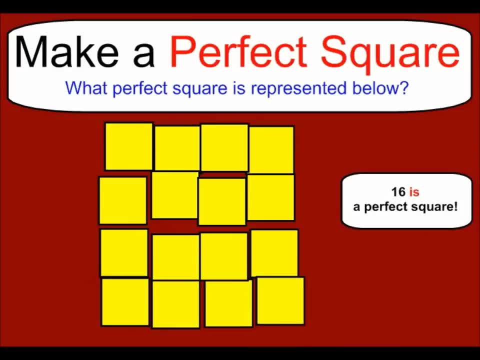 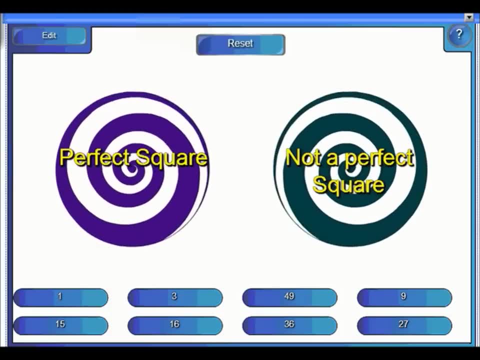 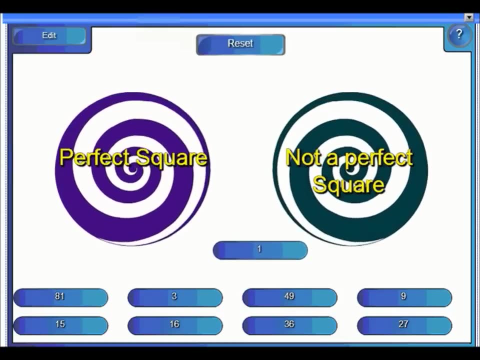 There we go. 16 is a perfect square. Now here's a little activity. I'm going to take these numbers and drag it into one of two vortexes, The number 1.. Do you think it is a perfect square? Is it a perfect square or not a perfect square? 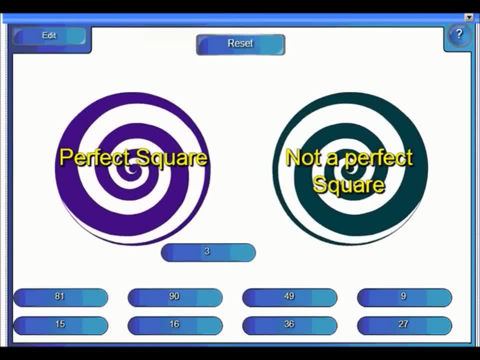 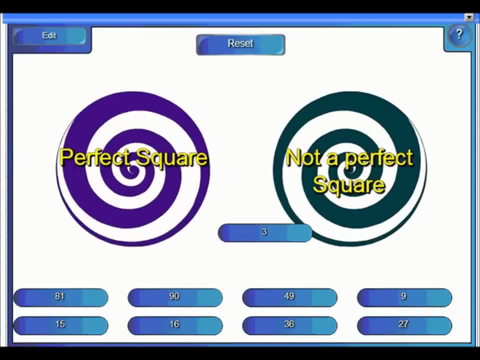 1 is a perfect square. What about 3?? Do you think it's a perfect square? Let's see if it is. No, it is not. 3 is not a perfect square. You can't make a square out of 3.. 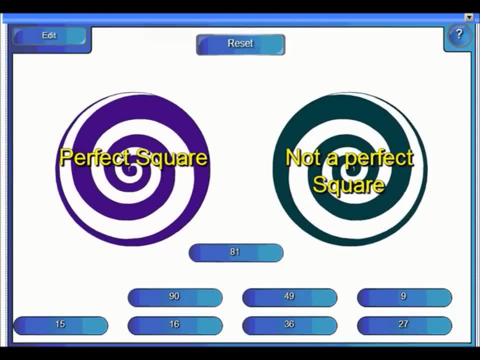 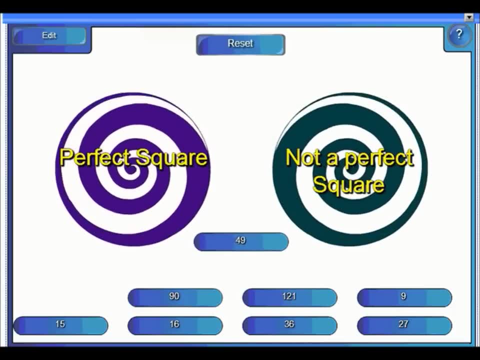 Is 81, a perfect square. Well, 9 times 9 is 81.. 9 squared is 81.. So, yup, it's a perfect square. What about 49?? Is any number squared 49?? Is any number squared 49?? 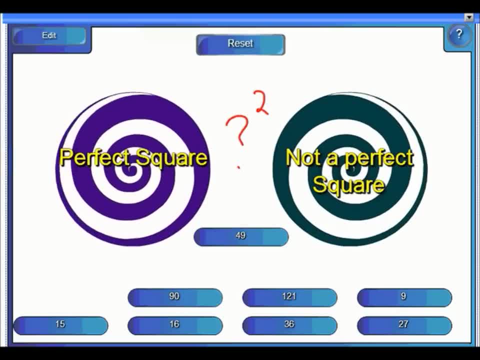 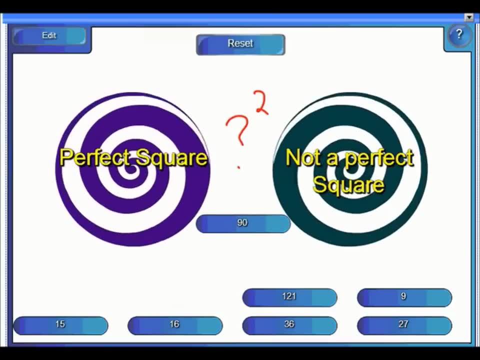 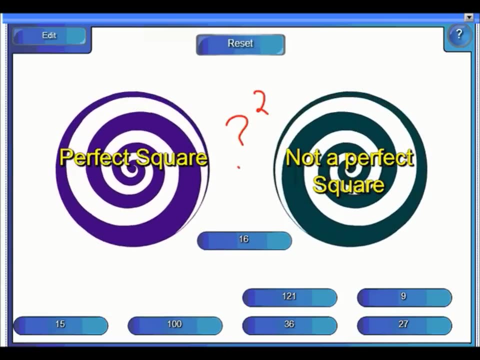 Is any number squared 49?? Yes, 7 squared is 49.. 49 is a perfect square. What about 90?? Is some number squared 90?? Nope. What about 16?? Is some number times itself 16? Yes, 4 squared is 16..